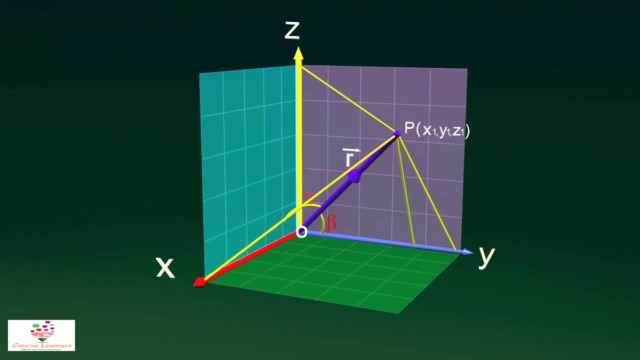 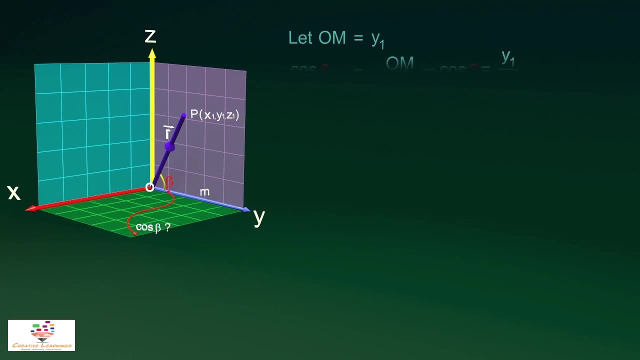 Direction cosines are the cosines of the angles between the line and the coordinate axis. Cos α, cos β, cos γ, denoted by l, m and n respectively, are direction cosines of OP. With the help of some simple mathematical operations one can find out the sum of squares of all three. direction cosines always remain one. 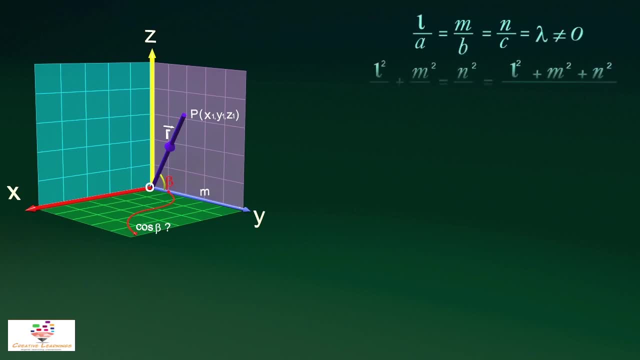 And if there exist a, b, c, such that then a, b, c are known as direction ratios and l m t are known as direction ratios and l m t are known as direction ratios. n are corresponding direction cosines. 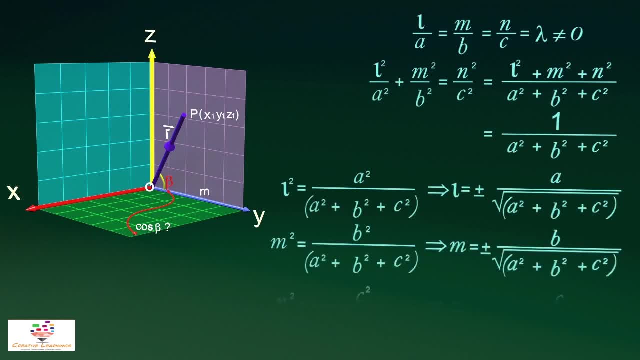 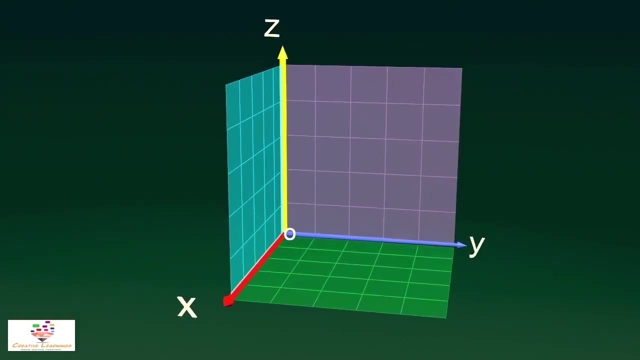 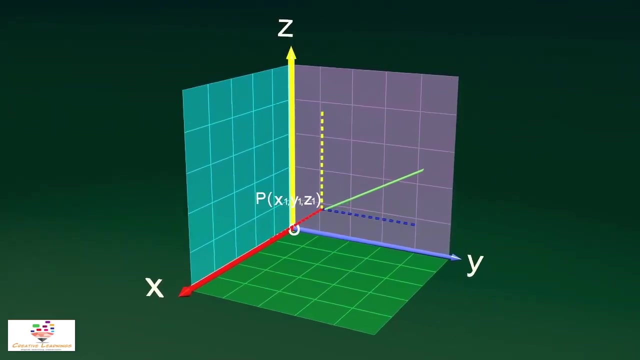 And one can also find the relation between direction cosines and direction ratios through some simple derivation. Now, if someone wants to find direction ratios of a line joining two points, P and Q, one can consider imaginary coordinate axes parallel to the original ones at any point. 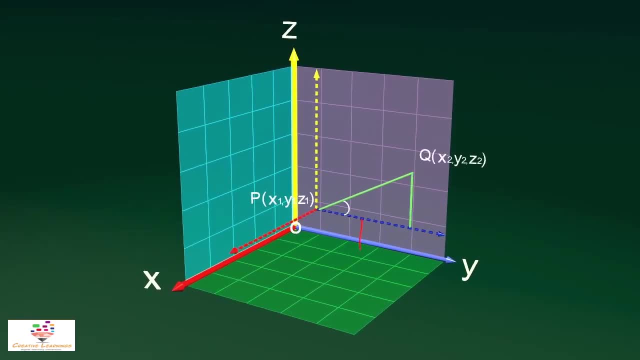 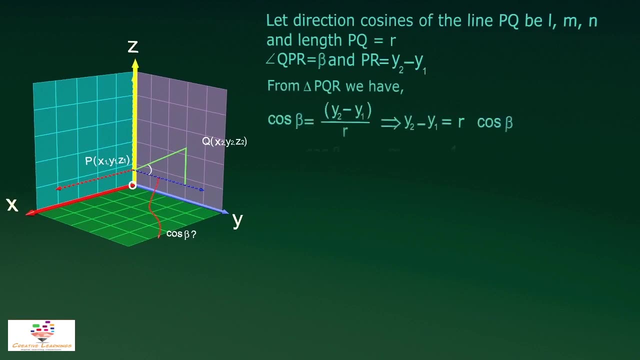 P or Q and can find the direction cosines similar to the previous one. In this example, we can find the direction cosines of the previous one, And the direction cosines of this direction are similar to the previous one. There are two ways to find the direction cosines of the previous one. 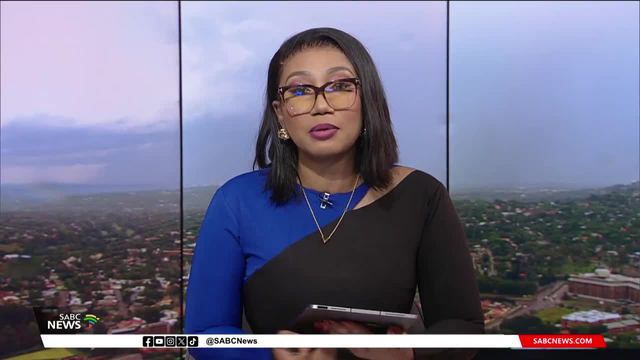 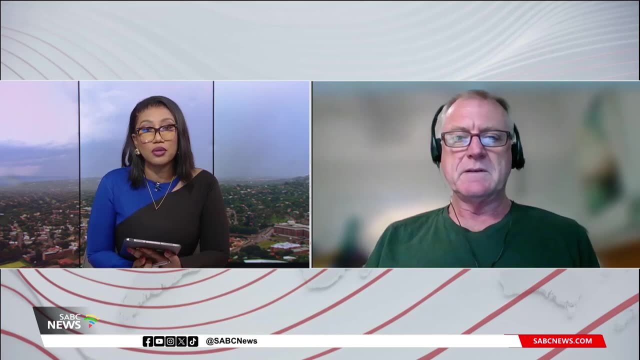 Now to discuss the inclement weather. we're joined by UCT climate scientist Dr Peter Johnston. Doctor, good afternoon and welcome to Full View. Good afternoon, It's a pleasure to have you with us Now, Doctor. we've all seen those images of the very strong winds and storms that are wreaking havoc in parts of the country. 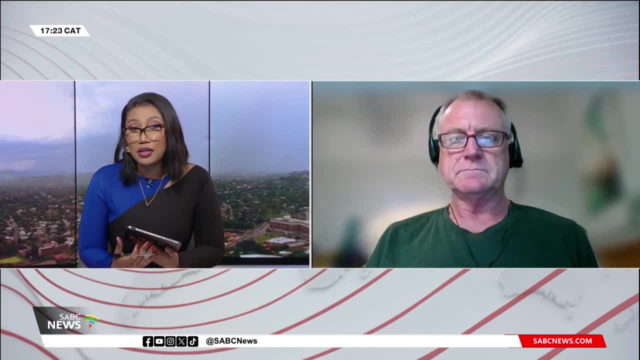 but particularly in the Western Cape. They're quite worrying. Now, in a statement by the South African Weather Service, it stated that the inclement weather is due what is called a cut-off low. What is a cut-off low and what weather conditions precede it? 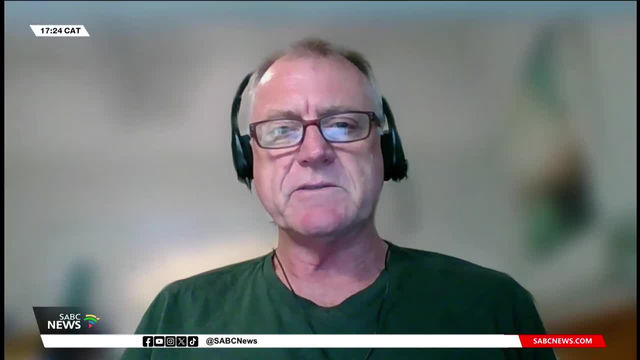 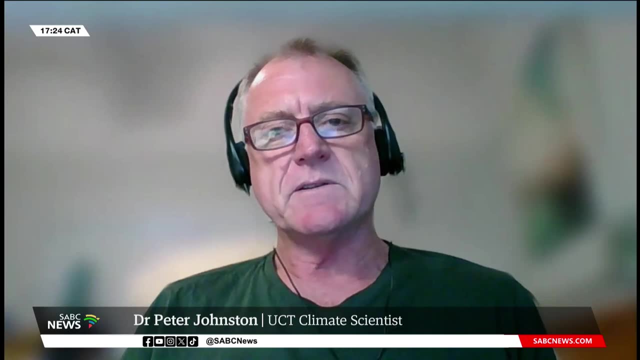 A cut-off low is a situation where a low-pressure cell is cut off from the belt of low pressures. If you live in the Western Cape, you're well aware that the rainfall comes from cold frontal systems which are at a certain latitude that we only get them in winter. That's when the sun is moving to the northern hemisphere and all the pressure belts are shifting up. So this low-pressure belt around about 30 degrees south in winter spins, It spins off little intense low-pressure cells in the upper atmosphere. Now, in the upper atmosphere means sort of 10 kilometres to 15 kilometres up in the sky. So that's why we call it cut-off. It's been sort of isolated and now it's gotten to the other side of the high-pressure, And what happens now is the high-pressure feeds moist air from the sea into that low-pressure, which is now extended down to the surface.